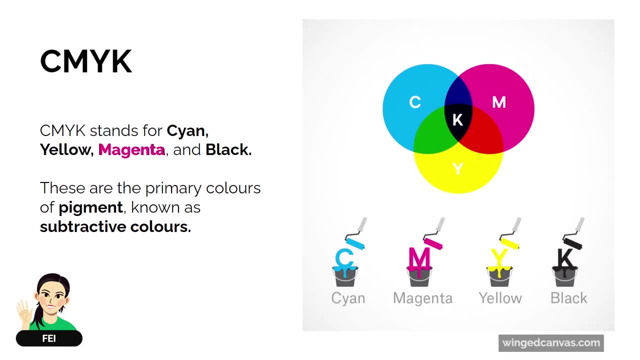 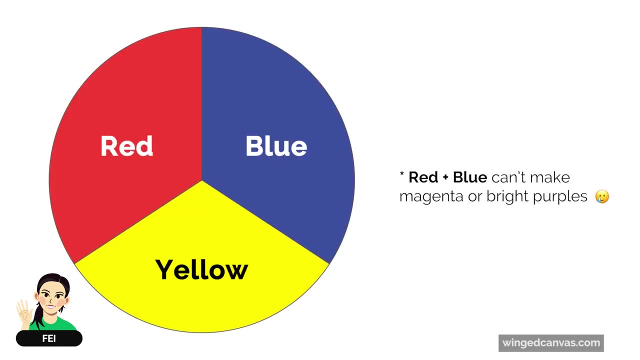 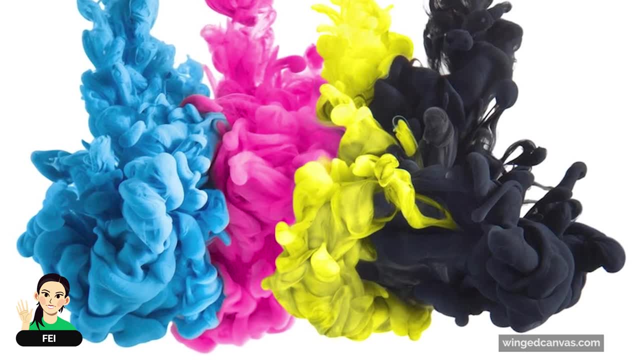 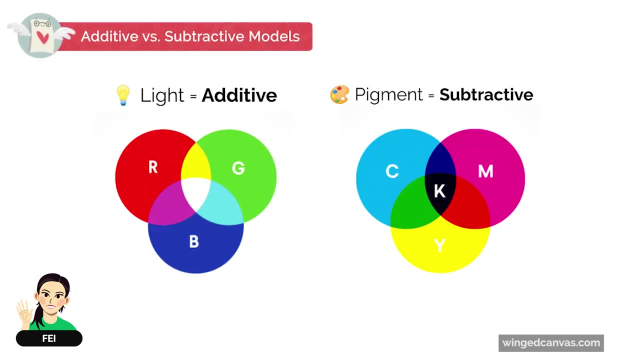 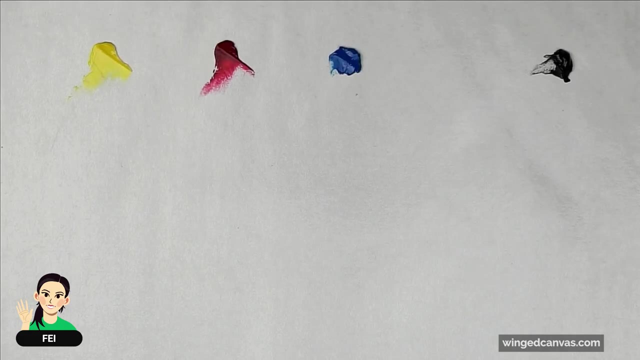 cyan, magenta and yellow are actually the purest primary colors that are found in pigment called a subtractive color wheel. Okay, So light is additive and pigment is subtractive. You'll notice that, like if you mix magenta, cyan and yellow together, you kind of get like: 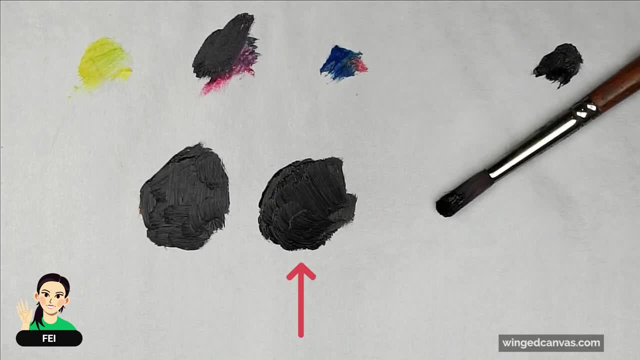 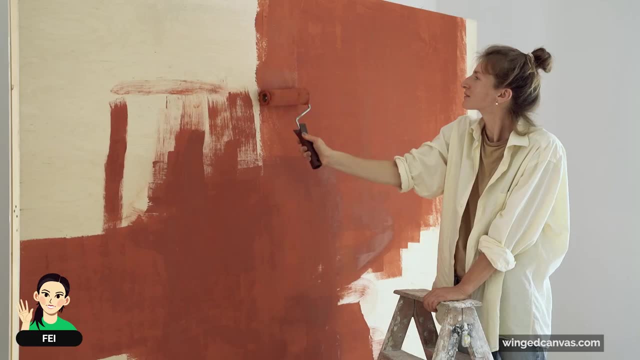 a dull black, not a pure black. So that's why they introduce a fourth color, which is black. So these are the applications that you would find CMYK in: you know house paint printer cartridges. you know colored powders, watercolor. 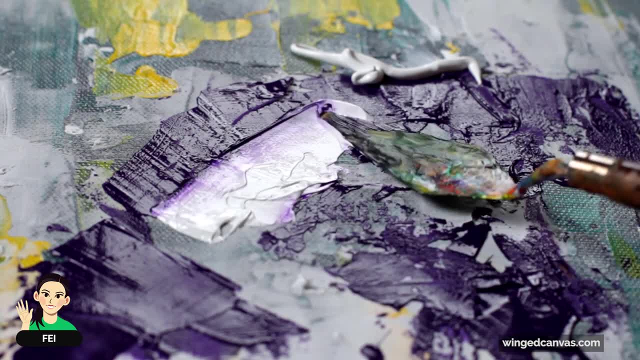 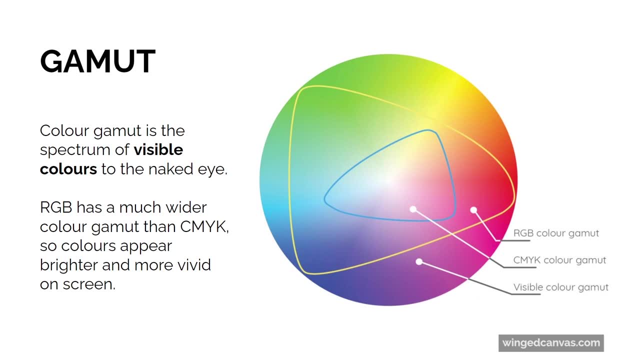 These are all made from organic and inorganic compounds. Okay, so, lastly, I'm going to talk a little bit about gamut. A gamut is the spectrum of visible colors to the naked eye. Okay, so what that means is we can only see a sliver of all of the colors that actually exist, right? 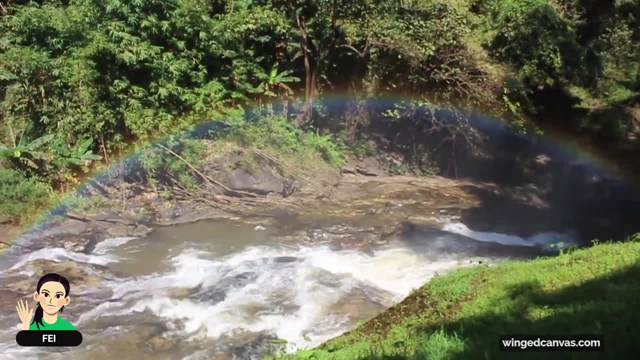 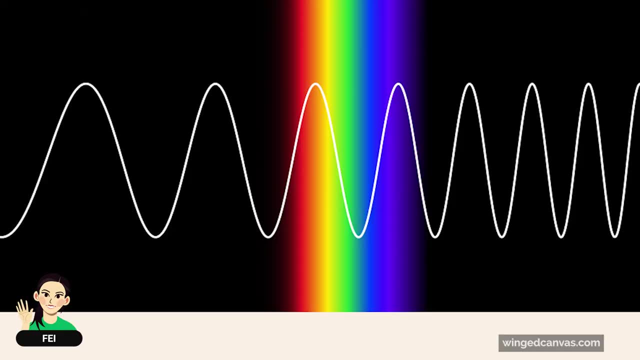 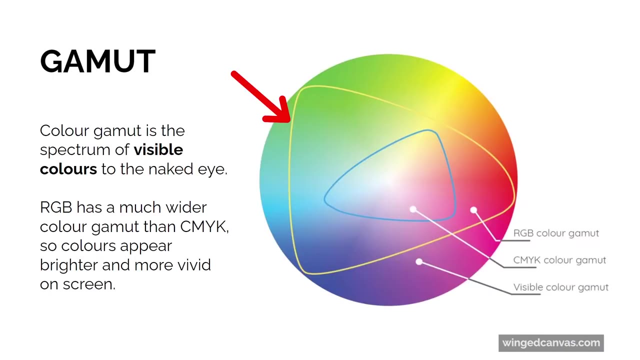 Our eyes can only see the colors of the rainbow, right, But the rainbow extends far beyond what our eyes can see. Just like, if you think about sound, right, We can hear sound waves, but we can't hear microwaves. And if you look at this yellow line here, this is the RGB color gamut. 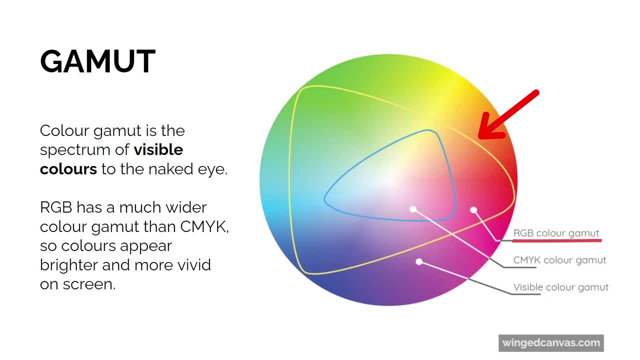 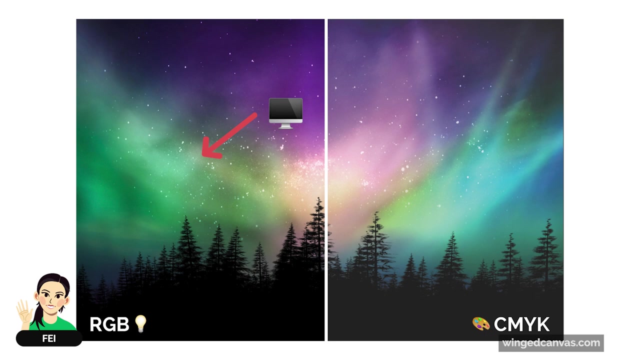 So the RGB color gamut is all of the colors that we are able to see from projected light, for example on a screen, And then the smaller triangle are all of color gamut in CMYK. What that means is if I have a beautiful image on screen right and I print it. if here it's additive and I'm seeing a very wide color range, and then I go to print it, the CMYK color gamut is a lot smaller.